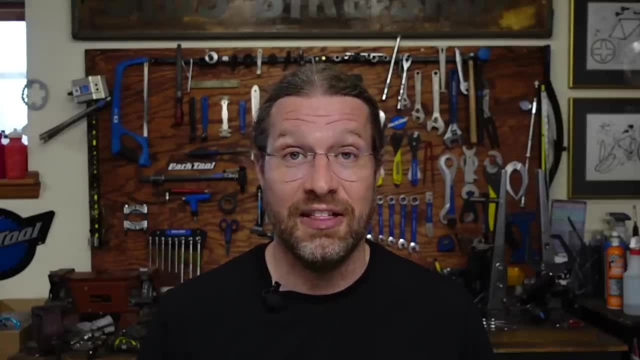 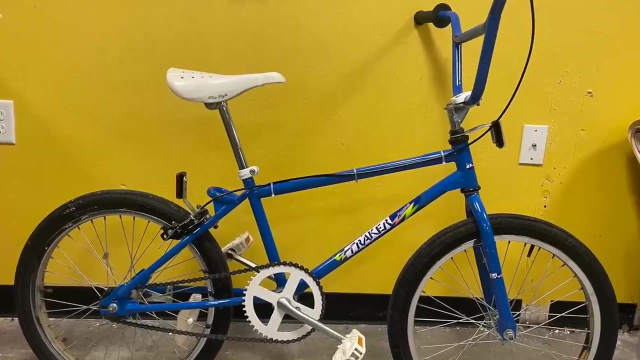 Even when my mom got her first bike from Gibbs in 1953, it was a reconditioned used bike. Even my first bike came from Gibbs in 1983. It was a Tracker Freestyle, a second-tier house brand of a regional parts distributor that nobody's ever heard of. 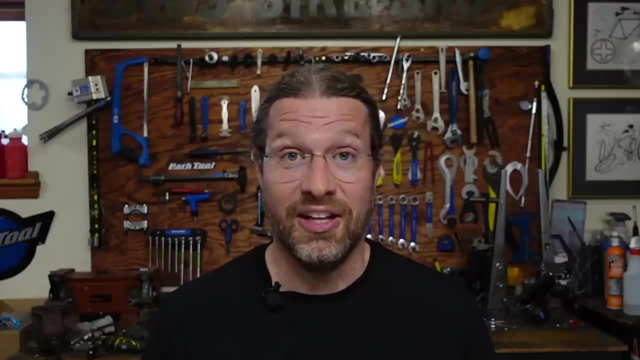 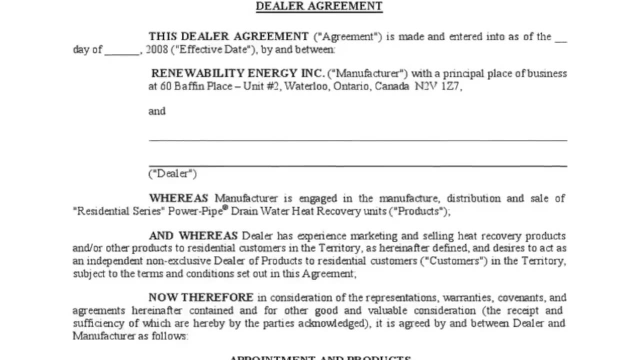 But around Gibbs passing in 1990, a Trek employee thought they'd try their hand as a Trek retailer in Lake Mills and opened the bicycle clinic. They lasted about five years before they ran into the same problems of never being able to meet the minimum purchasing requirements to remain a dealer. 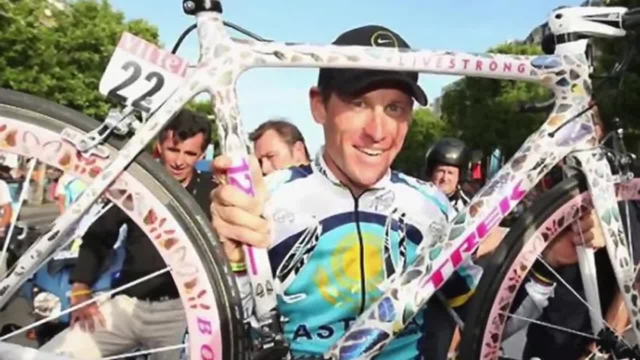 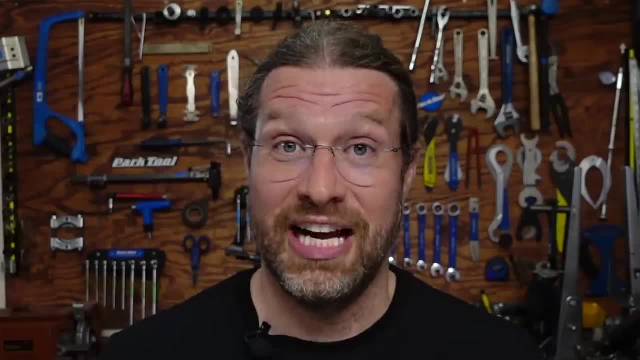 And so, as Trek signed on with the world's top racers and experienced stratospheric growth over the next 25 years, little old Lake Mills, Wisconsin, went shopless because you really got to be a special kind of stupid to try doing what I'm doing here. But I got something going. 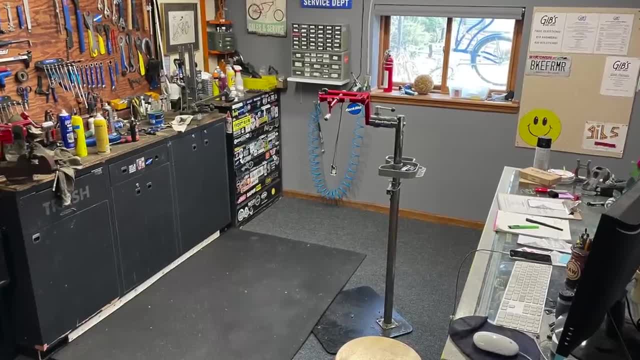 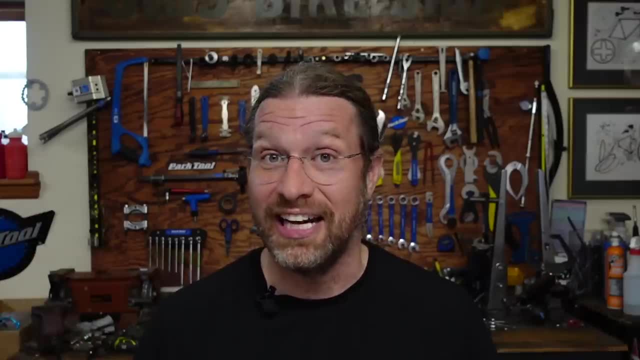 for me In my tiny little town, in my tiny little shop. I hear it all the time. I'm not a big biker and I don't need anything fancy like a Trek or anything like that. It's just regular people wanting to go for a bike ride, And it's not just here. Since starting this channel, I've learned: 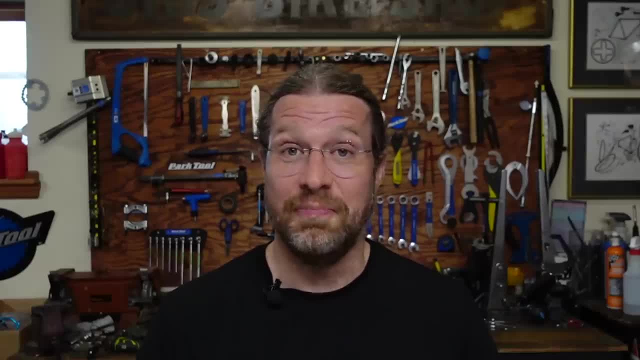 there are regular people across the globe that are really just turned off by all the fancy, overpriced bicycles and gear sold by the dominant cycling store model and would love to see a shift back to the smaller, independently owned, community-focused bike shops they remembered. 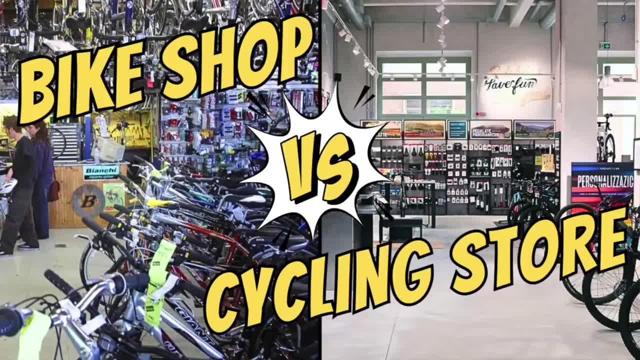 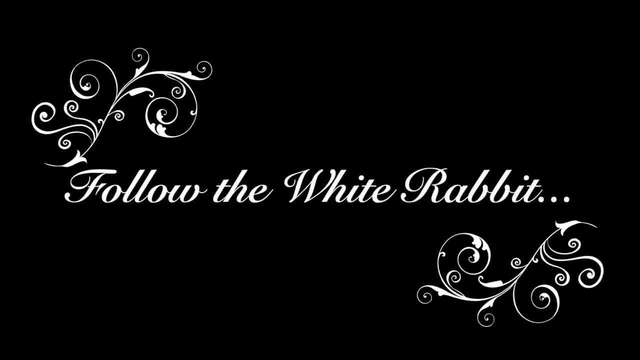 seeing when they were kids. So bike shops versus cycling stores- What the hell am I talking about? Well, follow me down the rabbit hole. If I had to distill it down to one simple sentence, it would be this: Bike shops provide. 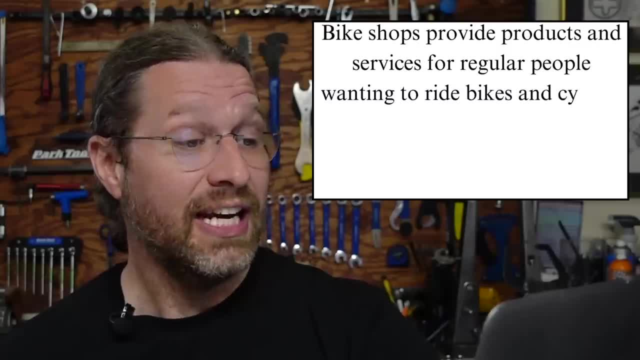 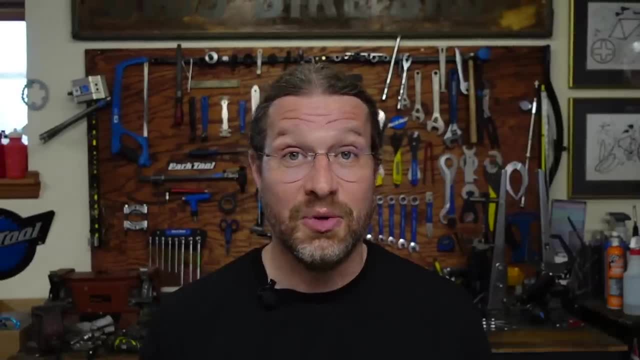 products and services for regular people wanting to ride bikes and cycling stores, create cyclists to consume novel bicycle products and services. to support industry trends And to dig into the nuance just a little bit more, I've written some really long run-on sentences to nail my point. 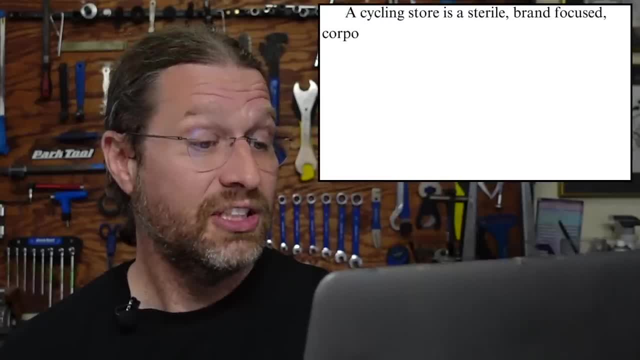 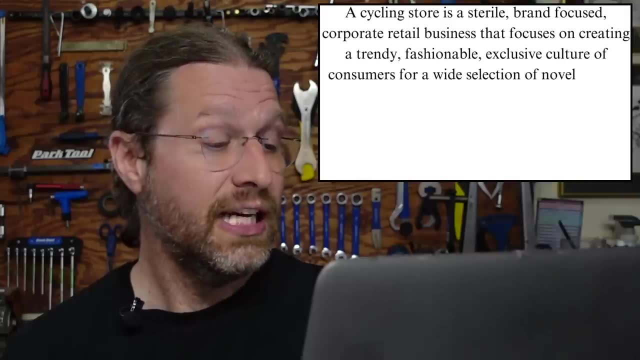 down further. A cycling store is a sterile, brand-focused corporate retail business that focuses on creating a trendy, fashionable, exclusive culture that is not just for the consumer. A cycling store is the culture of consumers for a wide selection of novel cycling products, by exploiting fitness and competition to ensure obsolescence requiring 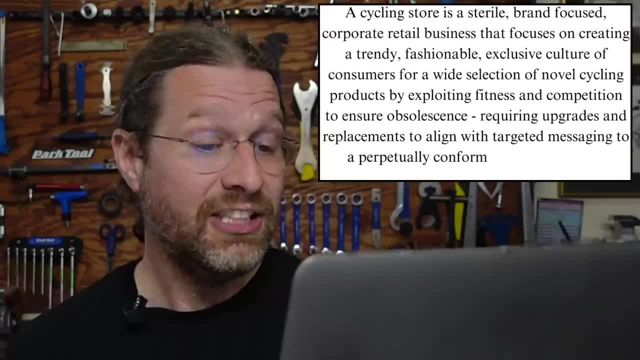 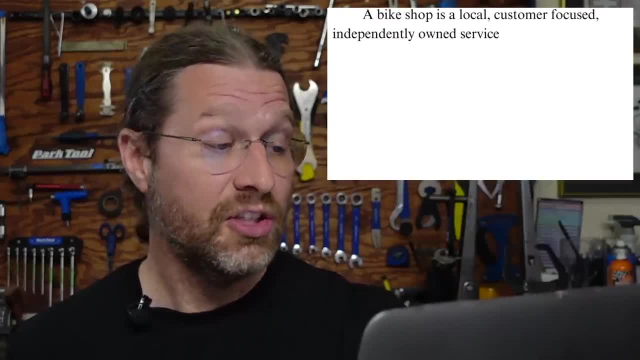 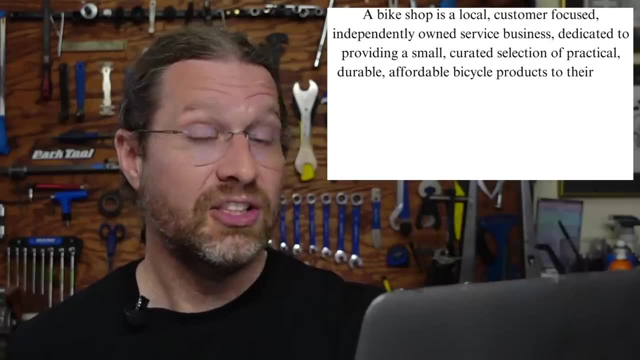 upgrades and replacements to align with targeted messaging to a perpetually conforming customer base. And a bike shop is a local, customer-focused, independently-owned service business dedicated to providing a small, curated selection of practical, durable, affordable bicycle products to their local communities by encouraging the use of bicycles in everyday activities. 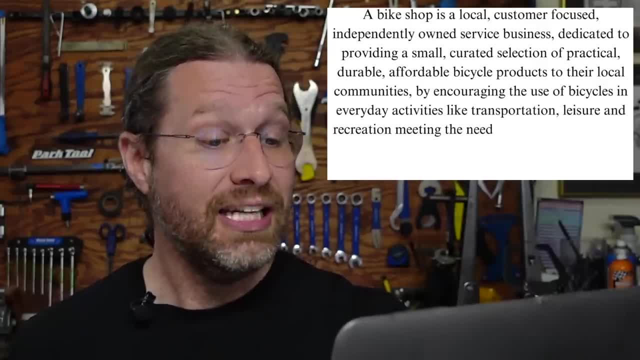 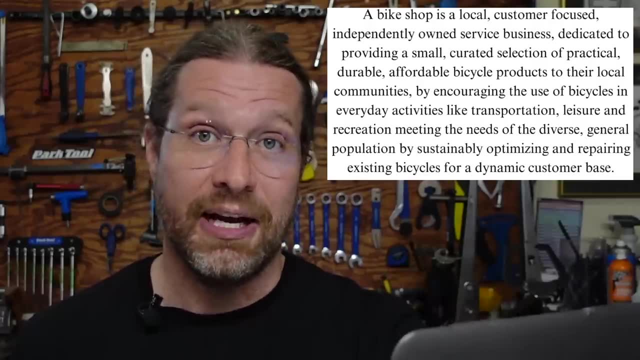 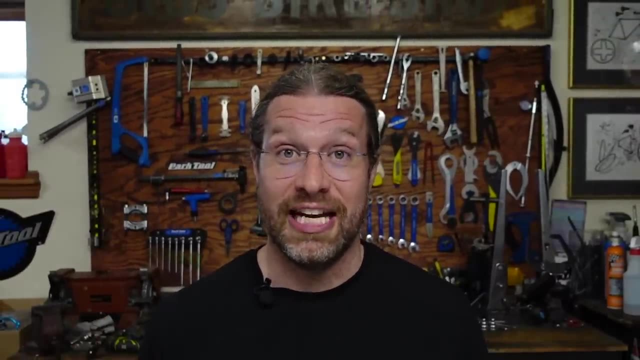 like bike shopping and cycling, And this is how a cycling store can help a diverse general population by optimising and repairing existing bicycles for a dynamic customer base. Whew, Now that's a mouthful For you simpletons. I've got some real-world examples. 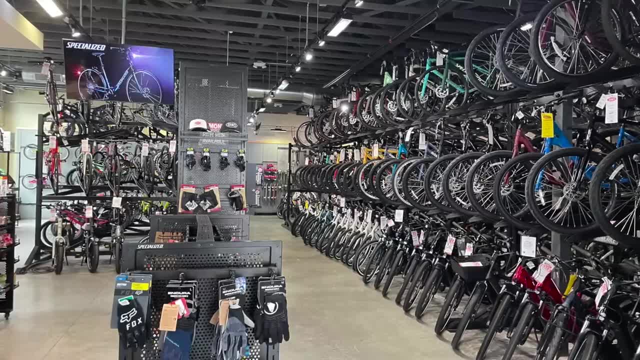 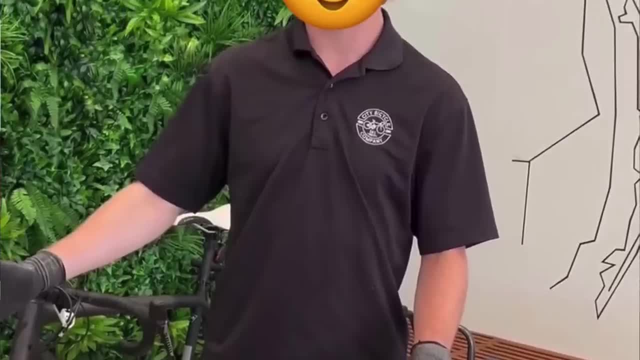 Now if it's a newer commercial location with clean floors and racks full of shiny new bikes ranging from $800 to $8,000, a clothing section and a well-groomed, fit gentleman with a buttoned-up shop shirt with a chest logo, it's a bike store that's not just for the individual. 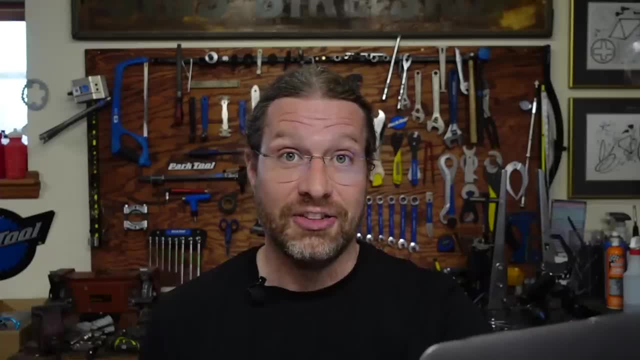 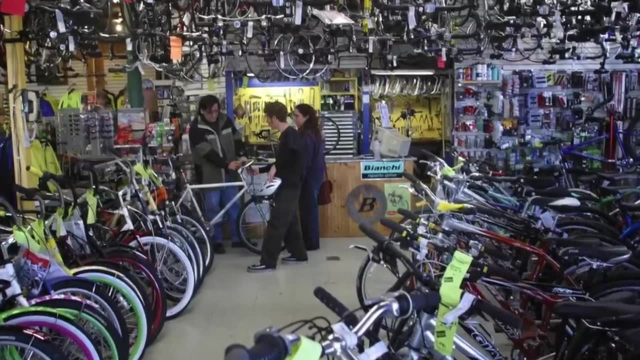 logo and flat brim SRAM hat greets you. you're in a cycling store, And if it's an old storefront with a faded sign, worn tile floors, with a row of $700 new bikes on racks above a row of $300 used bikes, some helmets stacked in a pile in the 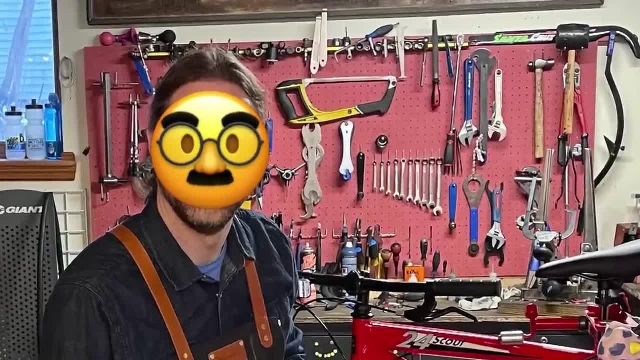 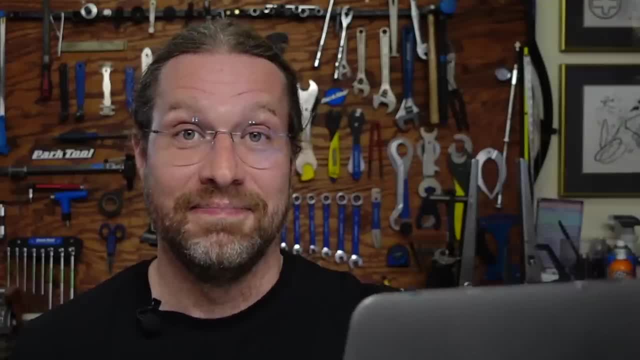 corner and a total dirt bag behind a dominant service counter in the back, with every inch of the wall covered in filthy tools and old stickers. congratulations, you found yourself a bike shop. I'm gonna simplify it even more, just so we fit in with today's world. Bike shops are for commies and 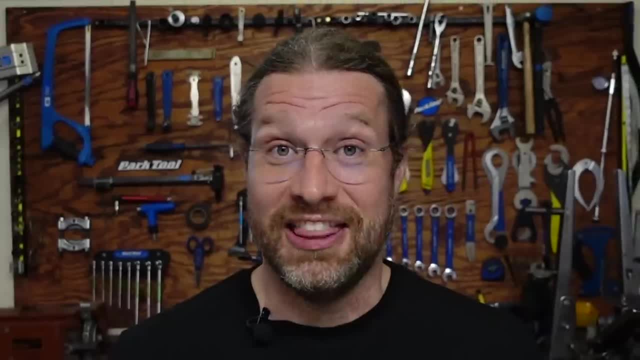 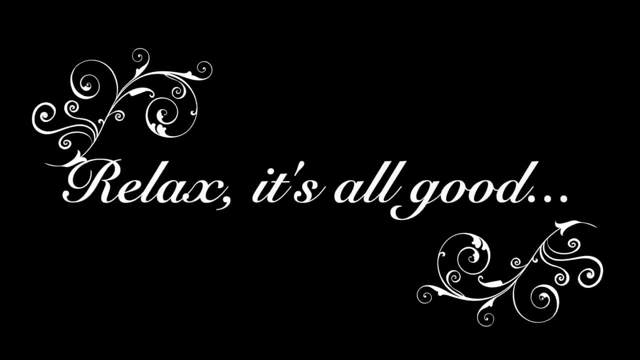 cycling stores are for capitalists. I suppose you think I'm about to tell you how it's gonna save the industry. huh Well, who am I to leave you hanging like that? Does the industry even need fixing? Probably not. I mean, bicycles are toys. 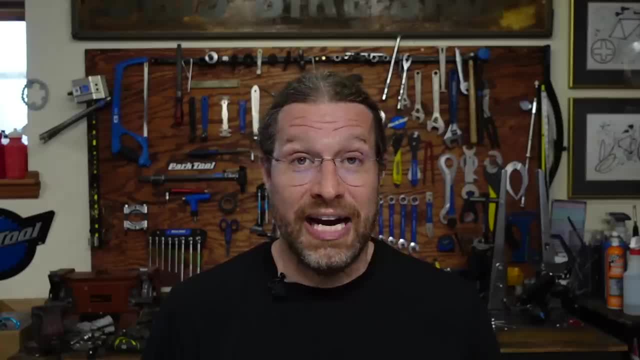 and fixing them is a hobby anyway, right, But with the dominant brands seemingly speaking out of both sides of their mouths and with no consensus of how we got here in the first place, we're going to have to figure out how we're going to. 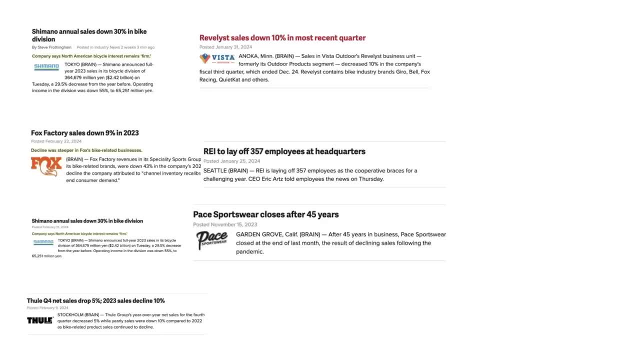 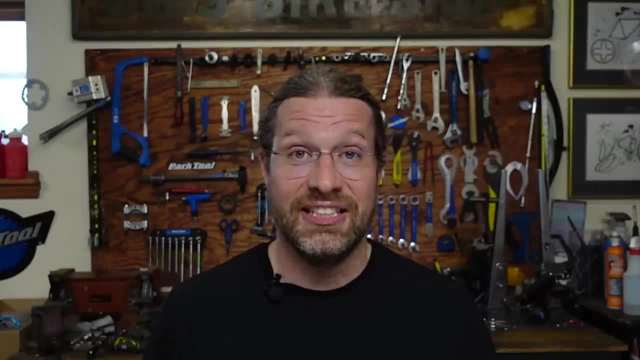 fix it. It's really no surprise that the industry has become so chaotic that people are calling it bikeageddon. Well, from where I sit, the past 25 years of tremendous growth and innovation in cycling has outgrown what the market can even understand. There are just way too many options out there, and big bike has. 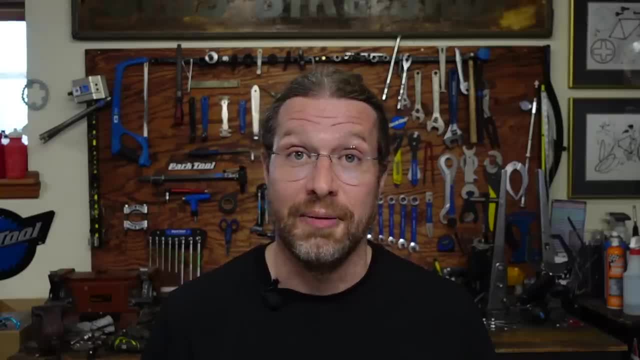 muddied the water so much that nobody wants to go swimming in the pond anymore. But let's be honest, I barely know how to fix bikes, let alone large bicycle corporations. I'm definitely not saying that I have the magic bullet that can. 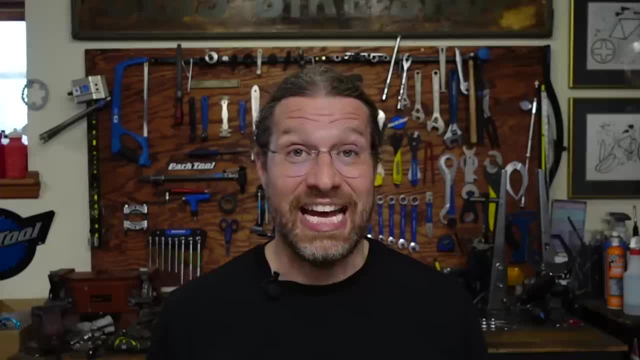 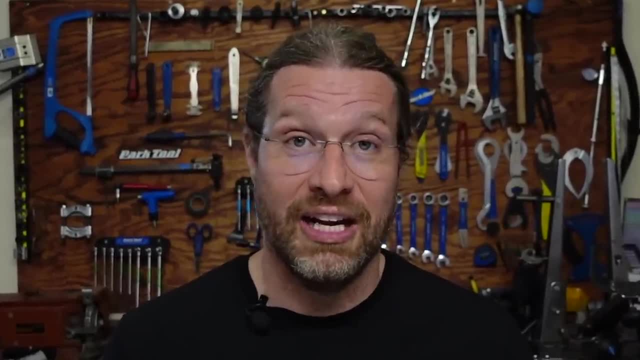 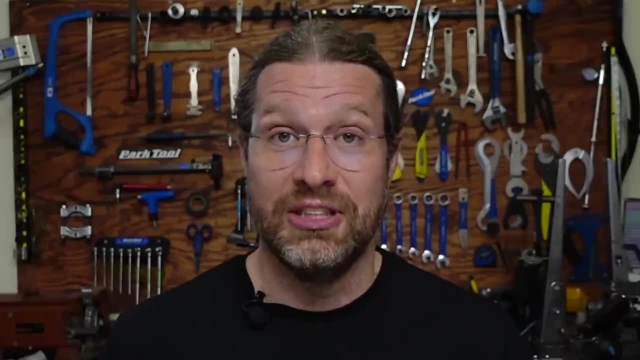 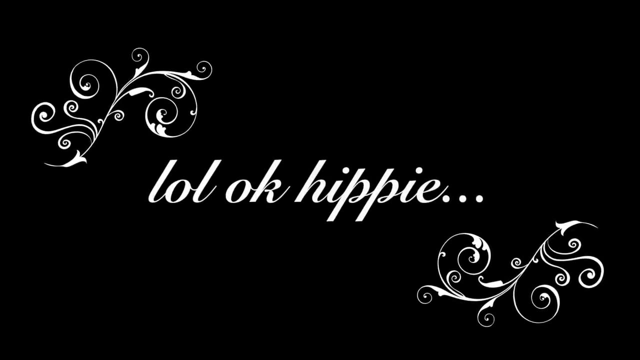 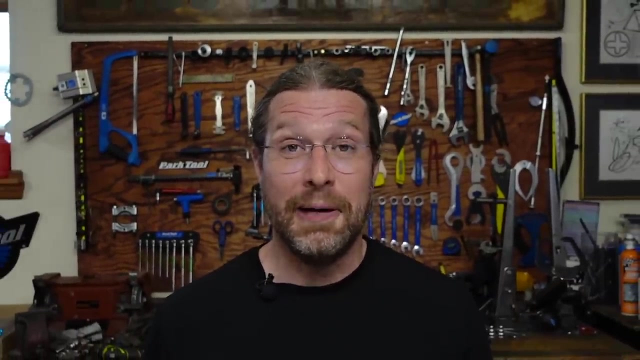 that bicycles bring into our lives and loosen our corporate grips and allow the local markets to decide what's right for their communities. When you try to be everything to everyone, it becomes too much for anyone. I feel like the big bike brands have made cycling into. 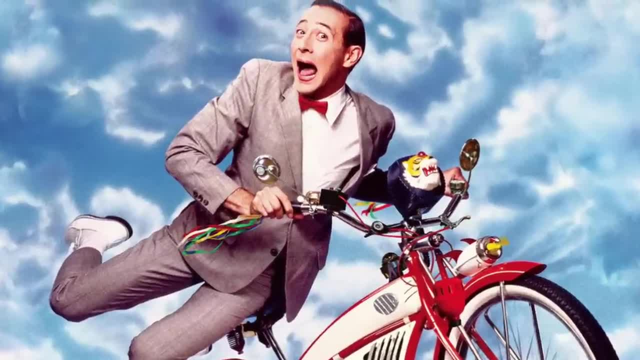 something that it's not. I feel like the big bike brands have made cycling into something that it's not. I feel like the big bike brands have made cycling into something that it's not. Riding a bike is supposed to just be fun, And when you make it so specialized and complicated, 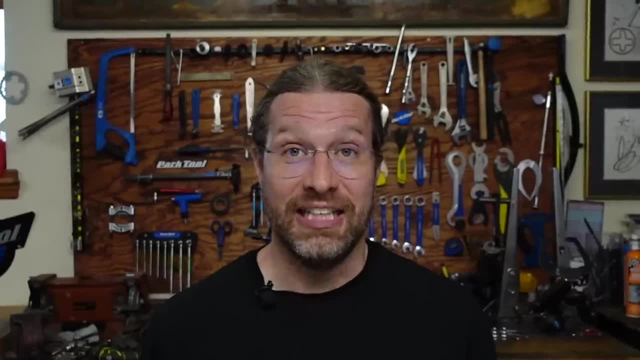 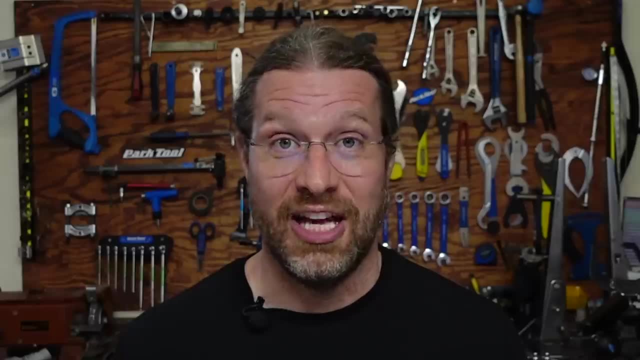 regular people aren't able to see it that way. I firmly believe that with a little bit of help anyone can enjoy riding a bike again. But when things get this complicated it makes it really difficult to sell that idea. I really like the idea of right-sizing things. 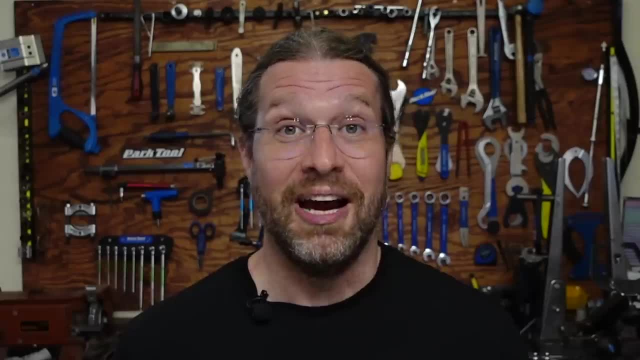 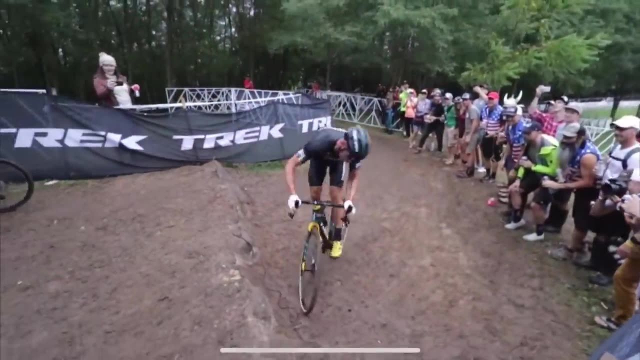 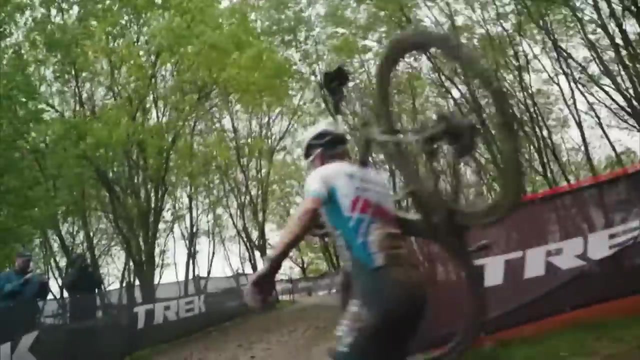 getting back to basics, because biking should be fun. I mean, seriously, what's not to love? It really doesn't need to be this complicated, right, Riding a bike is supposed to be fun, And when things get this complicated it makes it really difficult to sell that idea. I really like the idea of right-sizing things. 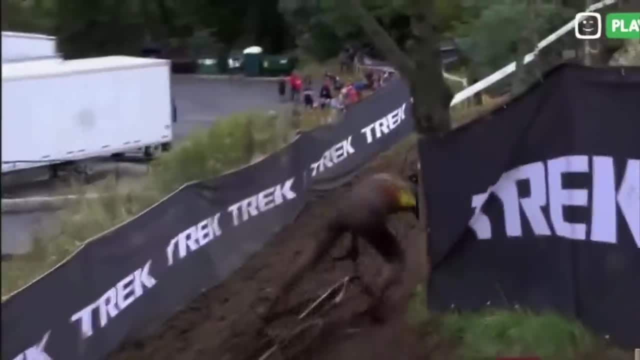 getting back to basic牛 hooking up all the time. Riding the bike is supposed to be fun. I really like the idea of right-sizing things, getting back to basic牛 hooking up all the time.